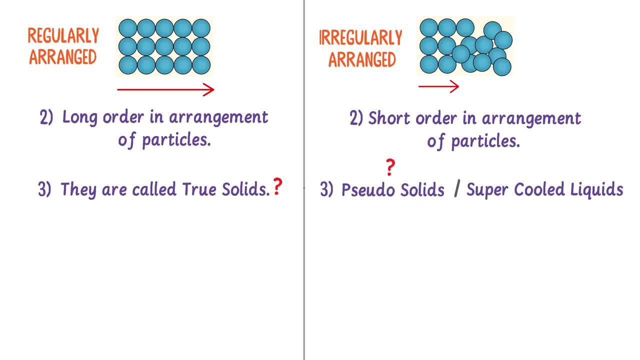 true solids and amorphous solids are called pseudosolids or supercooled liquids. Well, let me explain it. Giant solids are called true solids because they have true properties of solids, like they have regular arrangement of particles, they have long order and arrangement, etc. 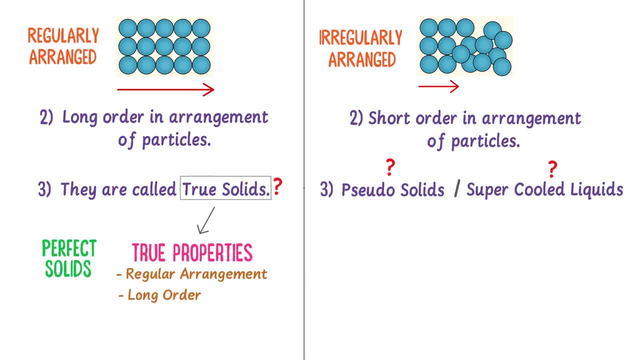 Personally, I call them perfect solids, While amorphous solids are called pseudo solids because they have fake properties of solids, like they have no regular arrangement of particles, no order and arrangement of particles, etc. Personally, I call them imperfect solids. Also, we call amorphous solids as supercooled liquids. 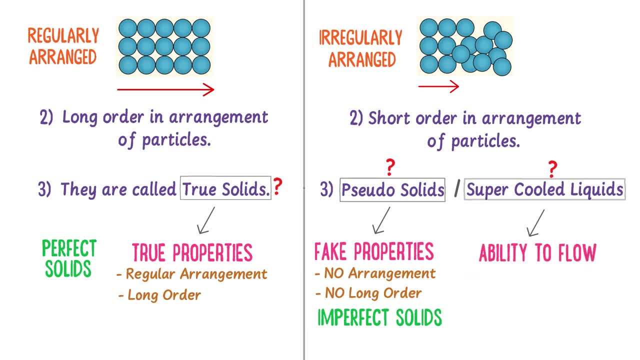 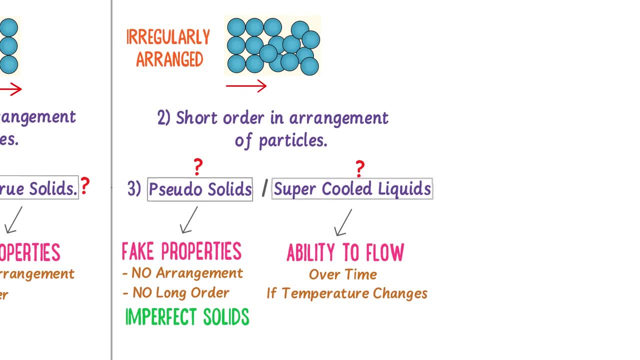 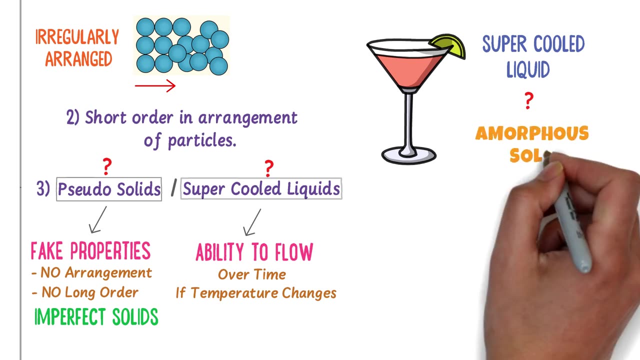 It is because they have ability to flow like liquids over time if temperature changes. Here let me teach you one of the most important questions of exam. Why is glass called a supercooled liquid? Well, glass is an amorphous solid. Molecules are irregularly arranged in it. 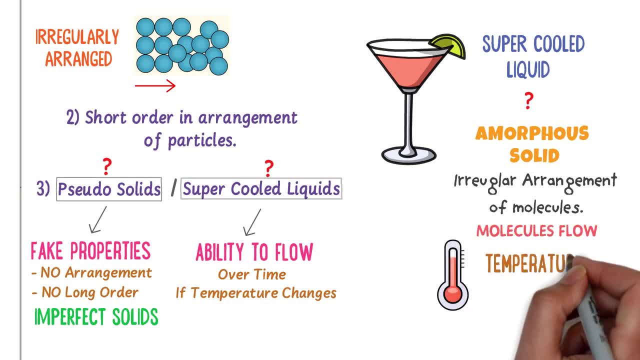 Due to which molecules can flow if there is change in temperature. For example, if temperature changes, then glass can flow like viscous fluid or honey if temperature is increased, So we therefore call it supercooled liquid. Fourthly, Crystalline solids have sharp melting point. 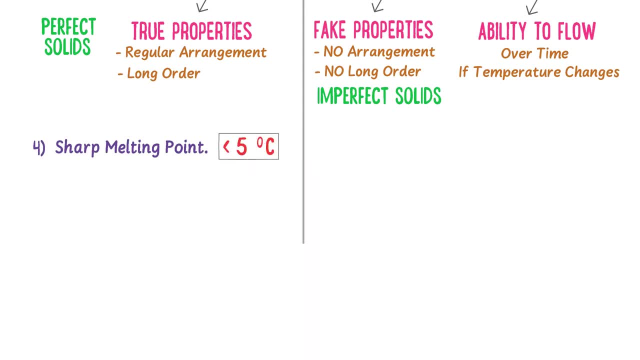 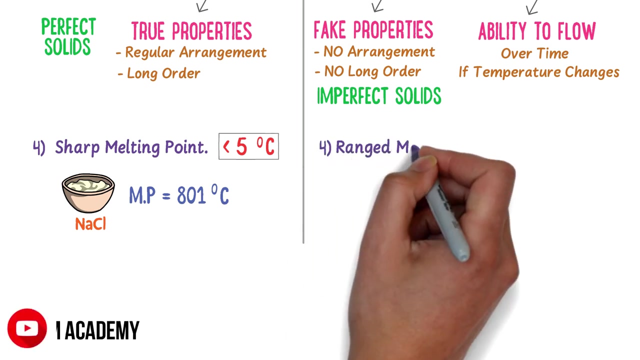 The range of melting point is less than 5°C. For example, the melting point of sodium chloride is 800°C. It may either increase or decrease by 5°C depending upon various factors, While amorphous solids have ranged melting point. 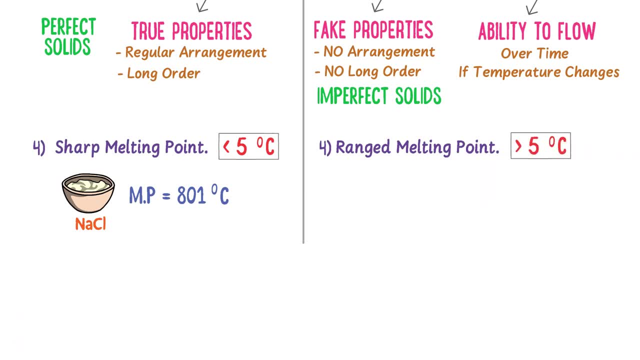 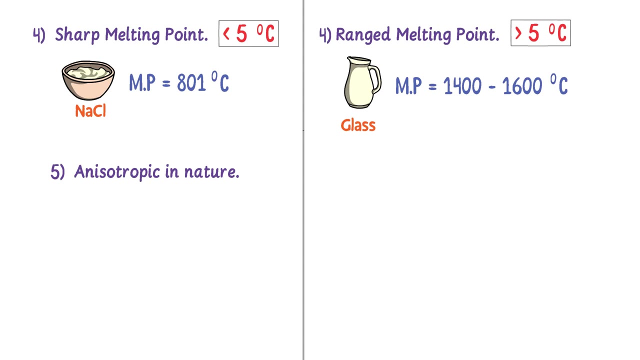 The range of melting point is greater than 5°C. For example, the melting point of glass is from 1400°C up to 1600°C. Fifthly, Crystalline solids are anisotropic in nature, While amorphous solids are isotropic in nature. 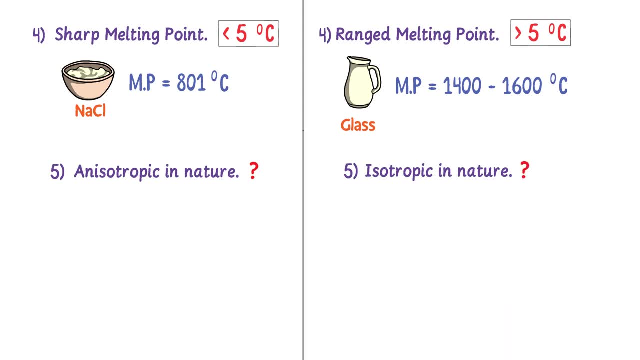 Do you know the meaning of anisotropic and isotropic property? Well, let me explain it. Anisotropic means that crystalline solids have different physical properties and different directions. For example, consider wood. The speed of light would be different in the wood and different directions. 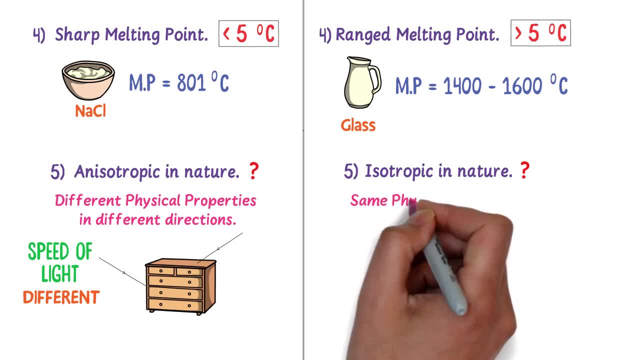 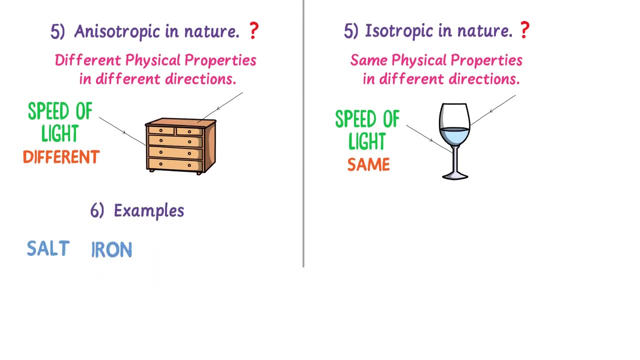 While isotropic means that amorphous solids have the same physical properties and different directions. For example, consider glass. The speed of light would be the same in all directions. Sixthly, the examples of crystalline solids are sodium chloride, iron, gold, sugar, etc. 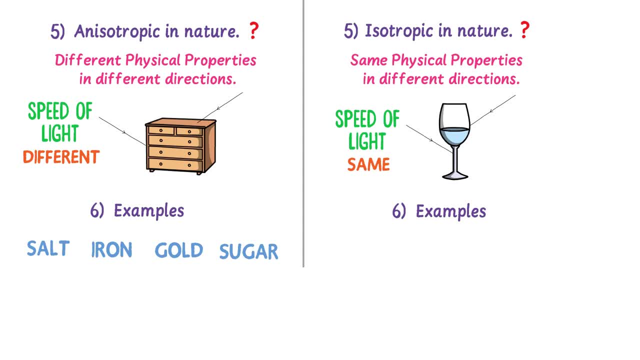 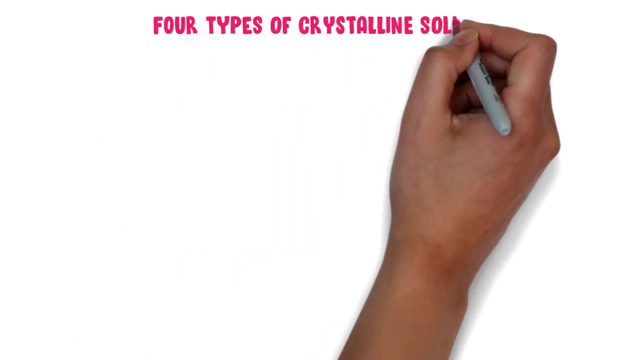 While the examples of amorphous solids are glass, rubber, wax, etc. Just note it down, all these important points about crystalline solids and amorphous solids. In any case, let's get back to the subject Now. let me teach you the four types of crystalline solids, because we have to study all about. 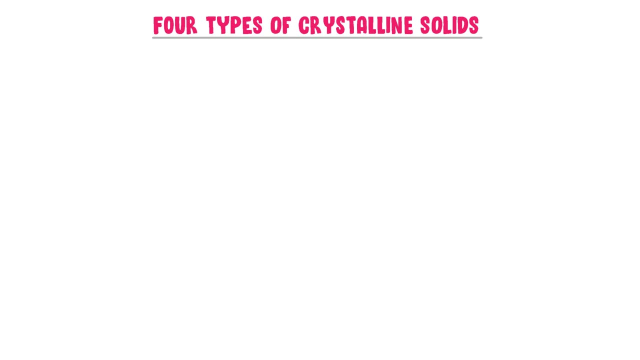 crystalline solids in our college course. The four types of crystalline solids are ionic solids, metallic solids, covalent solids and molecular solids. To learn all about these four types of crystalline solids, let me teach you my personal tray. 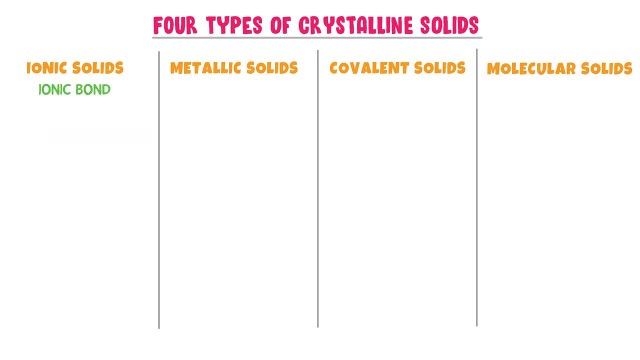 I always teach, as Ionic solids contain ionic bond. metallic solids contain metallic bond, covalent solids contain covalent bond and molecular solids also contain covalent bond. Now I will write the properties of each bond respectively. Ionic solids contain ionic bond, so their examples are sodium chloride, calcium carbonate, magnesium. 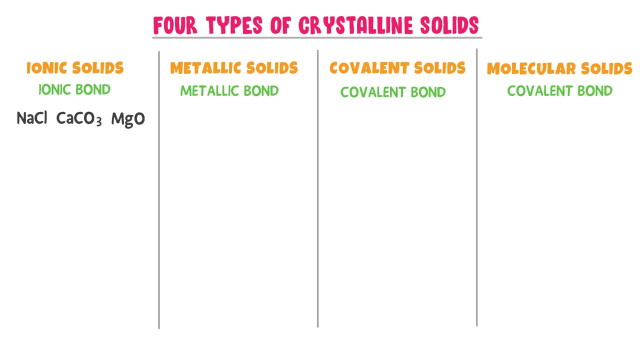 oxide, etc. Metallic solids contain metallic bond bond, so their examples are iron, gold and silver. Covalent solids contain covalent bonds, so their examples are diamond, graphite and silicon dioxide. Molecular solids also contain covalent bond, so their examples are ice, sugar and carbon dioxide. Now I will write all the